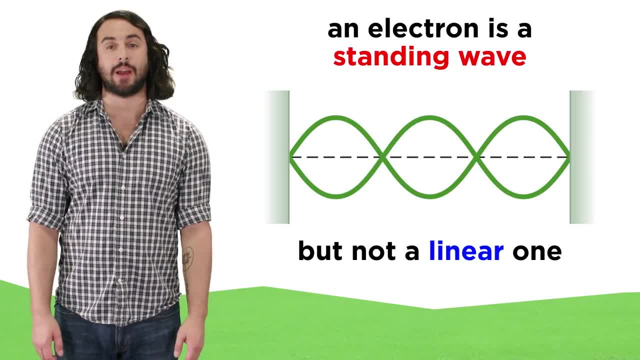 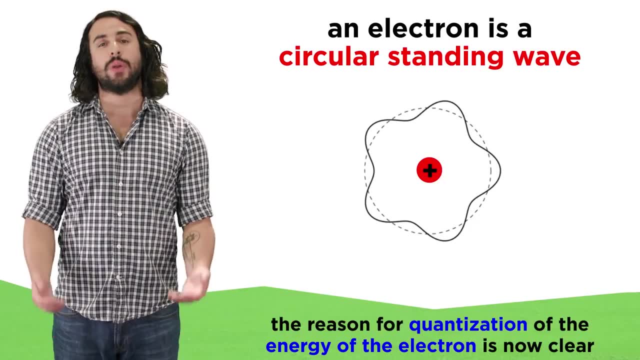 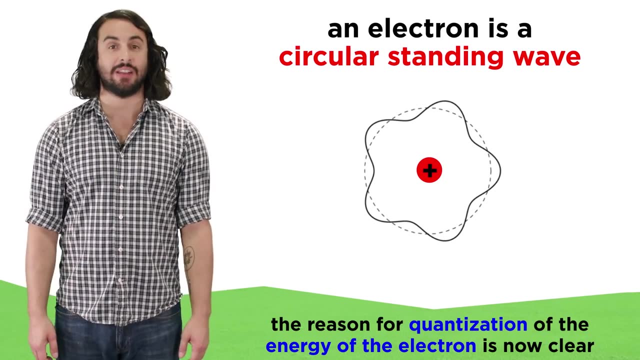 about in classical physics, except that, rather than something like a plucked guitar string, an electron is a circular standing wave surrounding the nucleus. If we understand this, it becomes immediately apparent why quantization of energy applies to the electron, because any circular standing wave 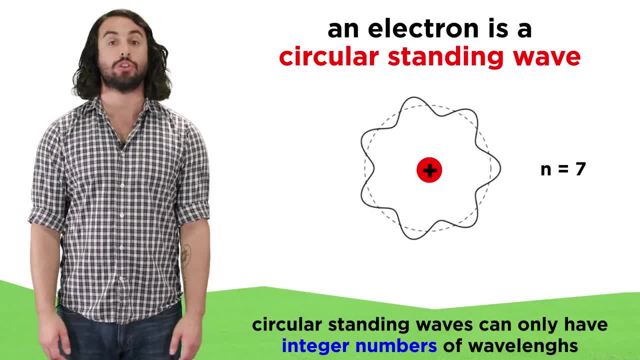 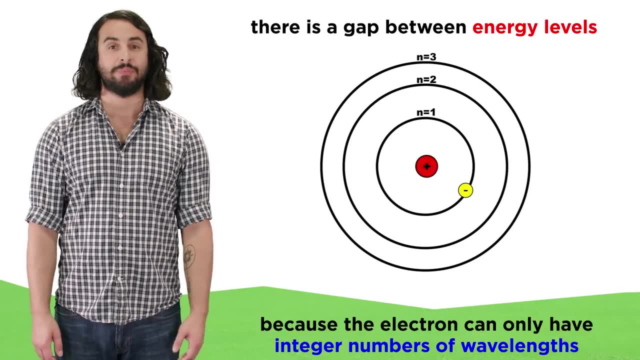 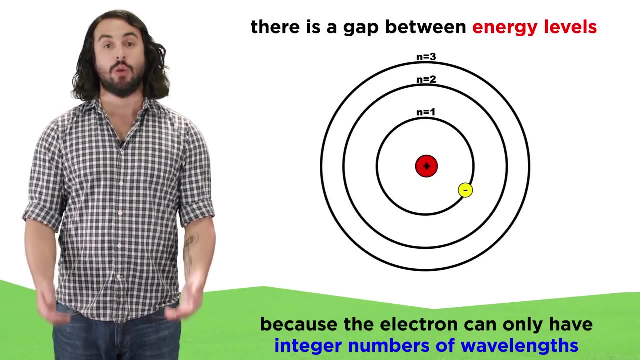 must have an integer number of wavelengths in order to exist. Given that an increasing number of wavelengths means more energy carried by the wave, we can see the Bohr model for the hydrogen atom begin to emerge, as we imagine a standing wave with one wavelength and then two, and then three and so forth. 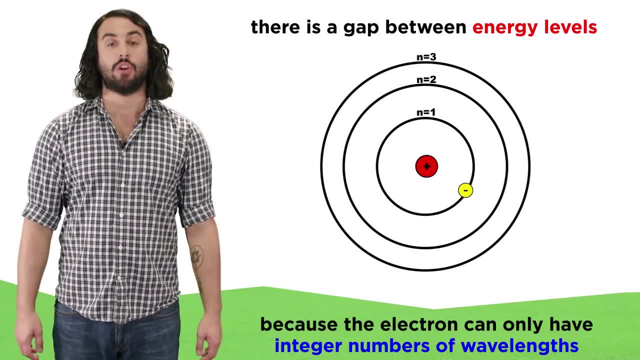 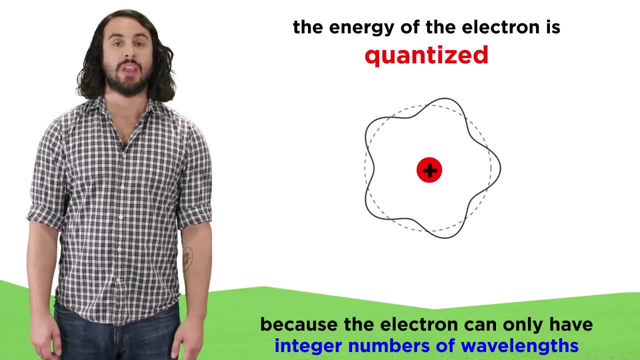 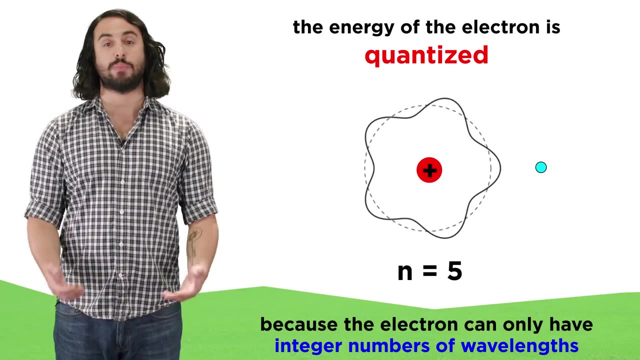 That is immediately obvious the reason that an electron in an atom can only inhabit a discrete set of energy levels. The circular standing wave that represents the electron can only have an integer number of wavelengths. When an electron is struck by a photon of a particular energy, this energy is 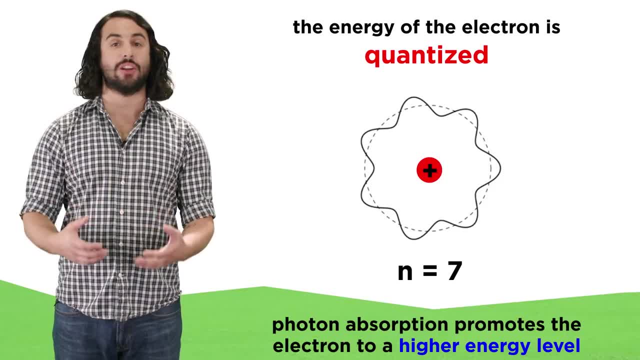 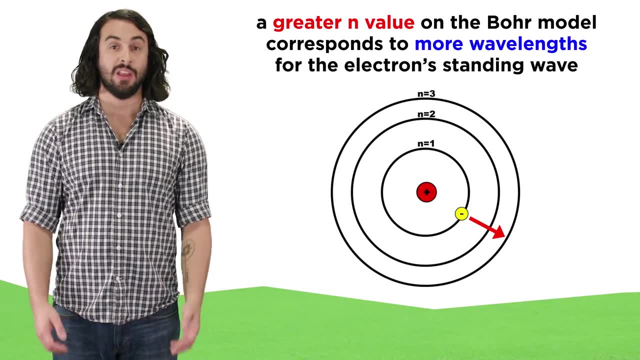 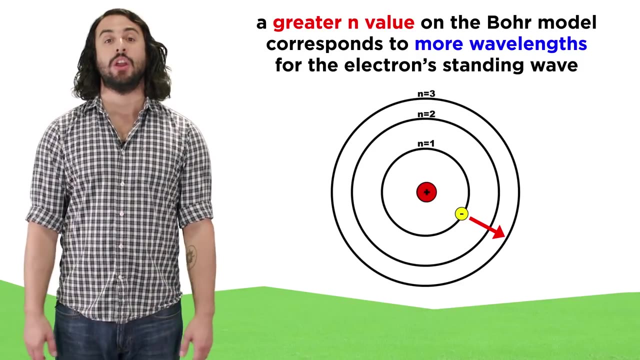 absorbed, promoting the electron to a higher energy state and increasing the number of wavelengths contained within the standing wave. This is why the electron goes to inhabit a higher energy level, and this is what is fundamentally occurring during electron excitation. Furthermore, it is the constructive 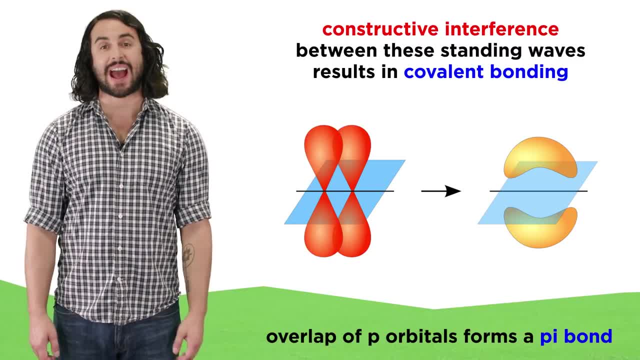 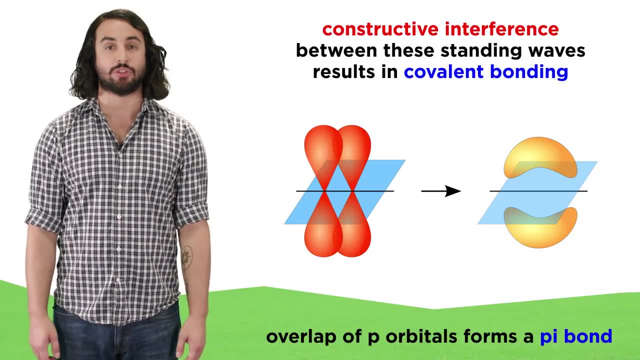 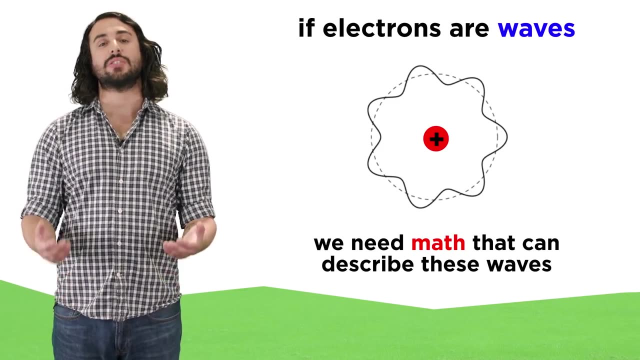 interference of these standing waves. that explains how orbital overlap results in covalent bonding. so we can enjoy a little more clarity in our understanding of chemistry thanks to modern physics. Once it was realized that electrons exhibit wave behavior, the physics community set out to find a 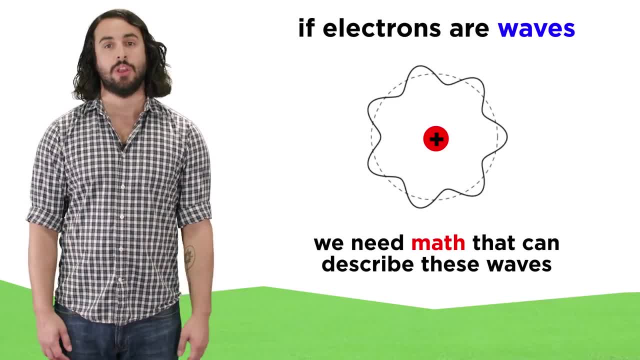 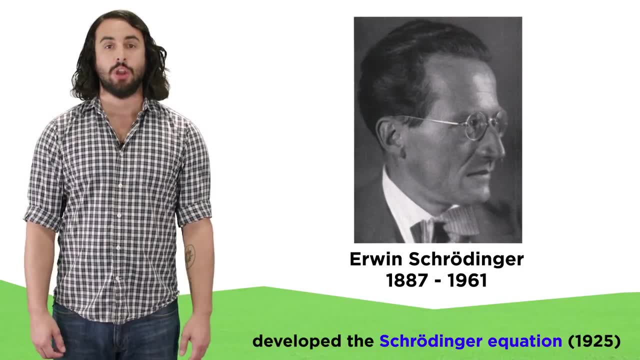 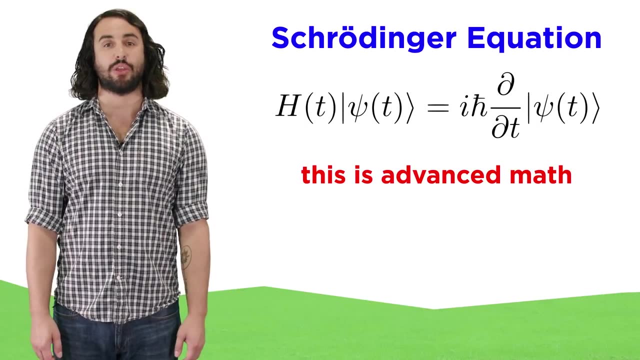 mathematical model that could describe this behavior. Erwin Schrödinger achieved this goal in 1925 when he developed his Schrödinger equation, which incorporated the de Broglie relation. This is a differential equation which utilizes concepts in mathematics that are beyond. 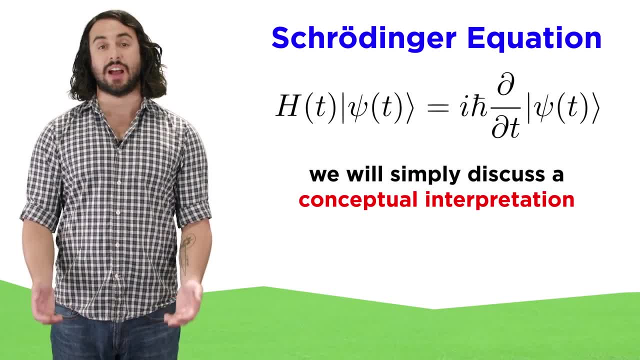 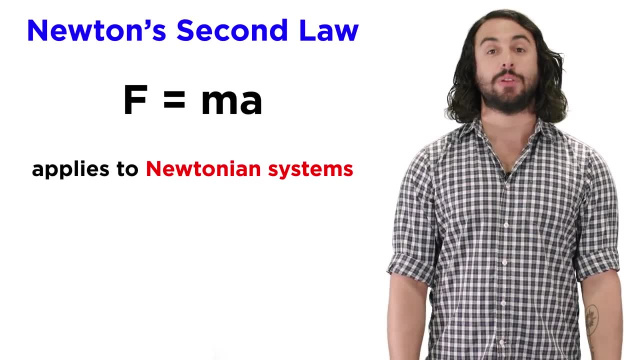 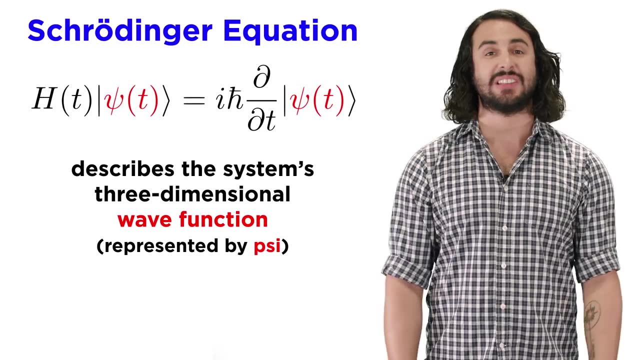 the scope of this series, but we can certainly discuss the conceptual implications of the equation. Essentially, just as F equals ma applies to Newtonian systems, the Schrödinger equation applies to quantum systems by describing the system's three-dimensional wave function. 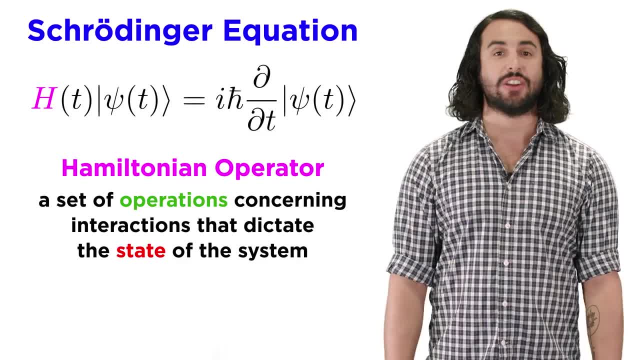 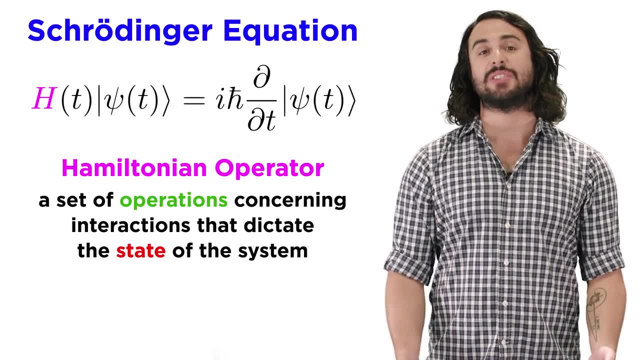 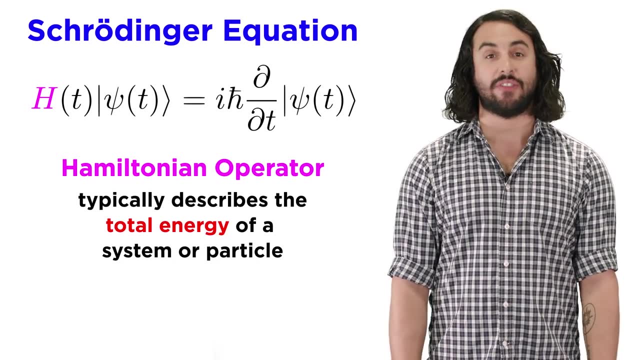 represented by the Greek letter psi. In this equation, this term is called the Hamiltonian operator, which is a set of mathematical operations that describes all the interactions that are affecting the state of the system, which can be interpreted as the total energy of a. 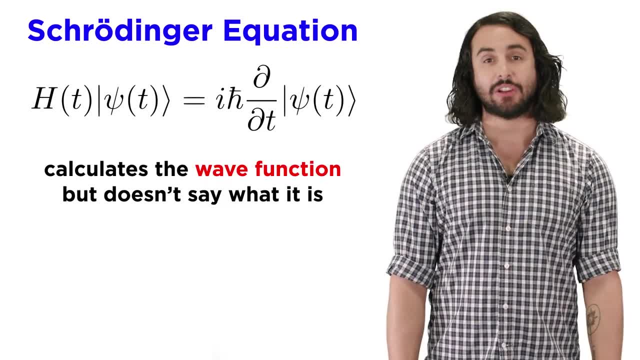 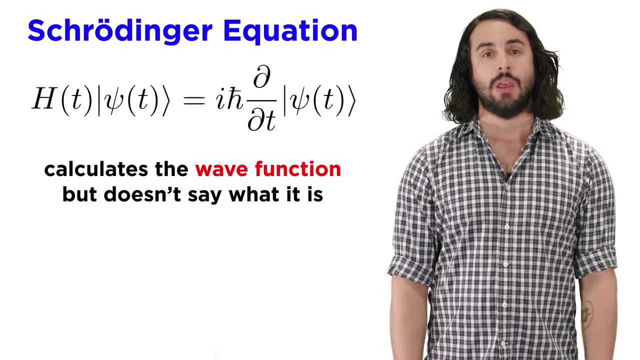 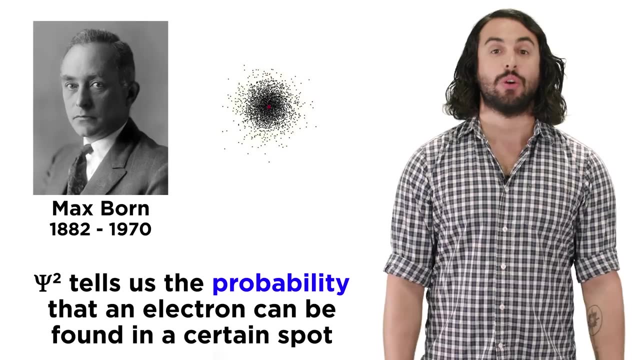 particle. But while the Schrödinger equation can calculate the wave function of a system, it does not specifically reveal what the wave function is. Max Born proposed that we interpret the wave function as a probability amplitude where the square of the magnitude of the 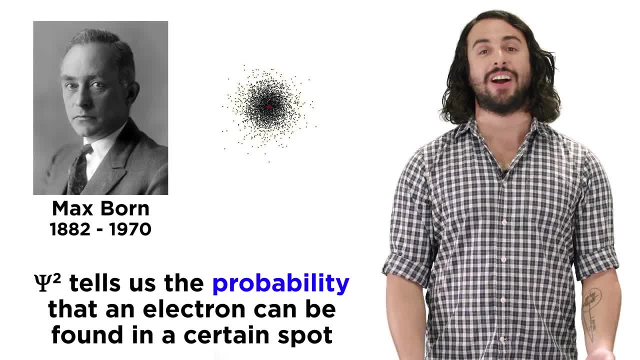 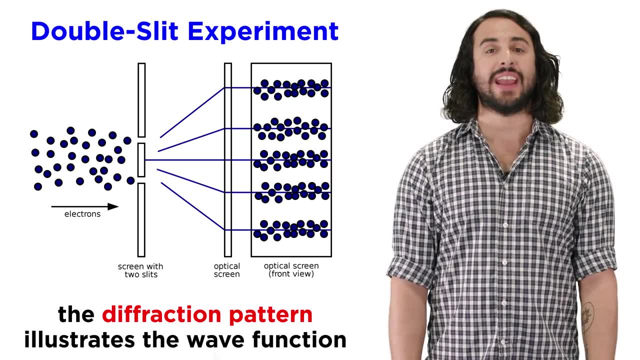 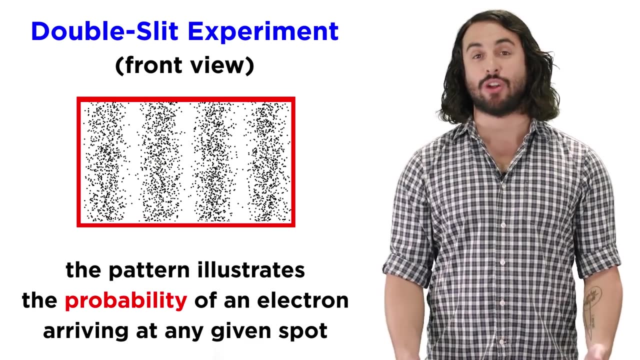 wave function describes the probability of an electron existing in a particular location. Looking back at the double-slit experiment, we understood that theượng 은 the diffraction pattern as illustrating this wave of probability. The pattern is not the electron itself. it is the probability that an electron will arrive. 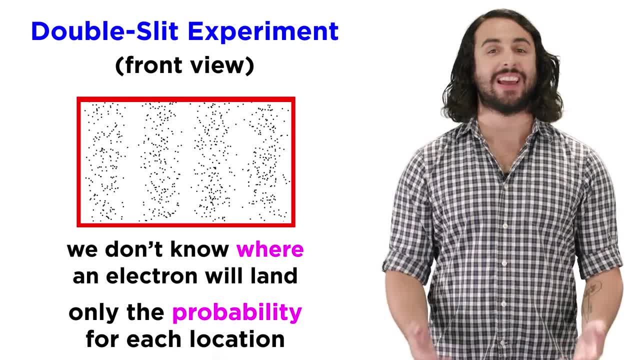 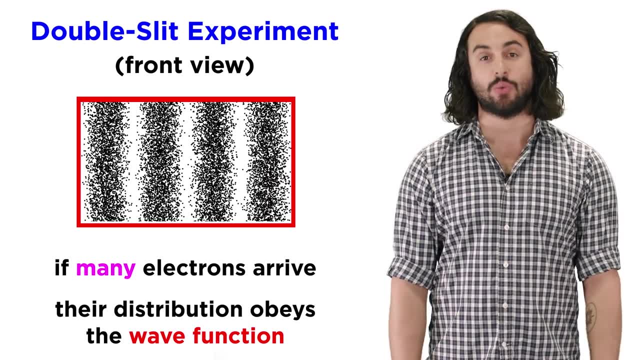 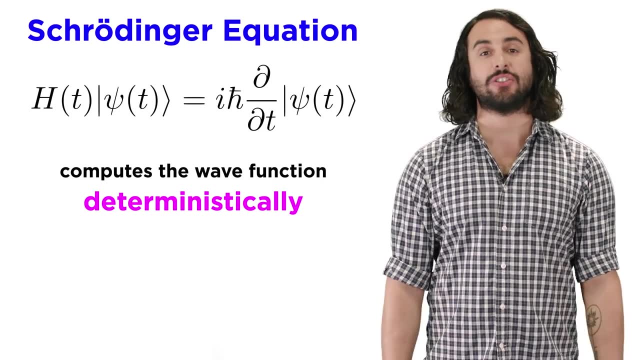 at each location on the screen. We can't predict where one electron will go, only the probability that it will arrive at a particular location. If many electrons arrive at the screen, it becomes apparent how their distribution obeys the wave function. So the Schrödinger equation does compute the wave function. 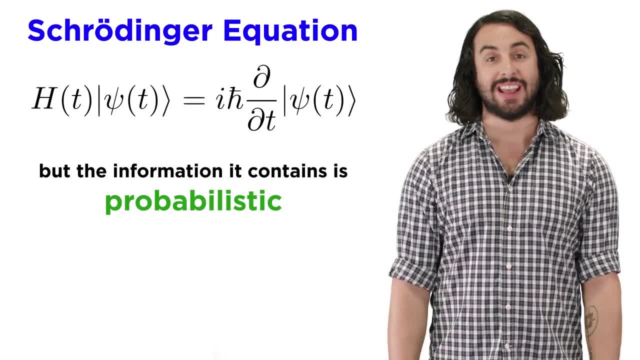 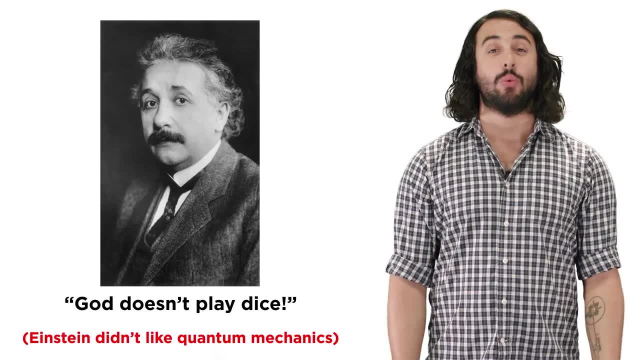 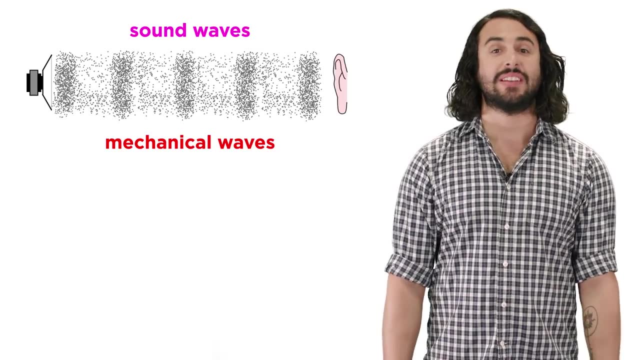 deterministically, but what the wave function tells us is probabilistic in nature. This idea that nature is probabilistic on the most fundamental level was a lot for the scientific community to handle at the time, and still is for some. So just the way, sound waves are mechanical waves and light. 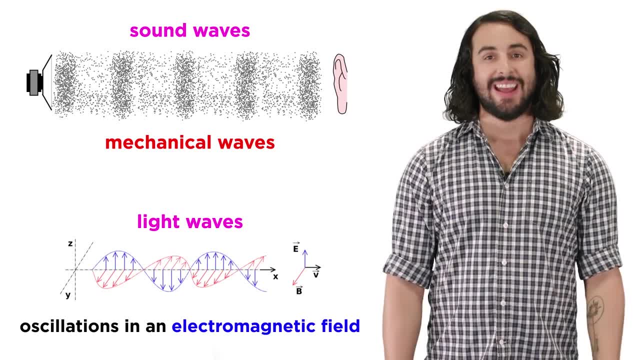 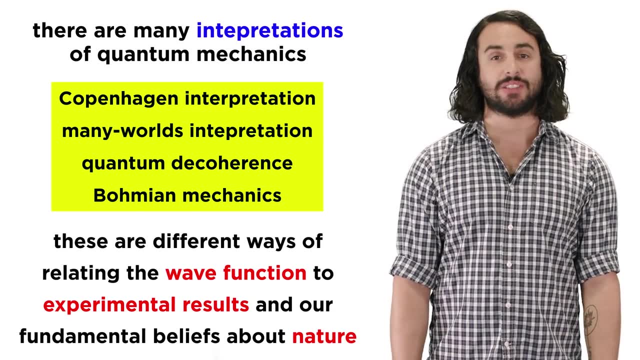 waves are oscillations in an electromagnetic field. an electron can be centro-directional, or it can be side-directional, or it can be top-directional, and an electron can be considered a cloud of probability density. There are many such interpretations of quantum mechanics, which involve different ways of viewing. 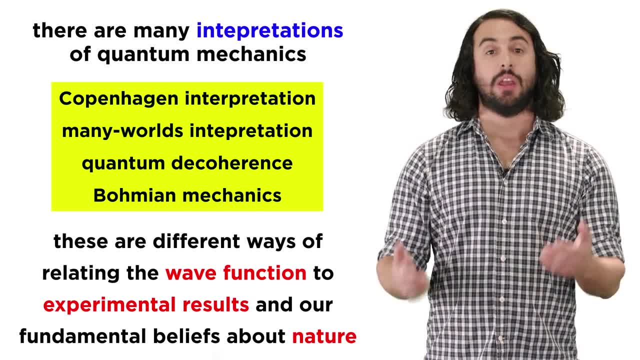 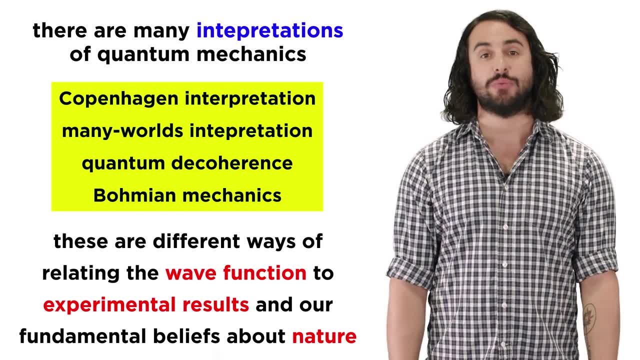 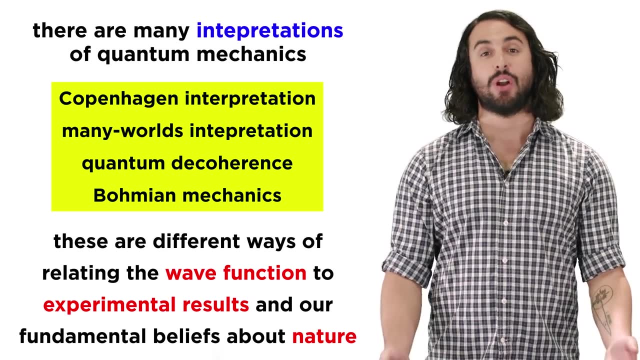 the relationship between the wave function, experimental results and the nature of reality, and there is still no firm consensus as to which view is correct, be it the Copenhagen interpretation, many worlds interpretation or a number of others. But before you choose a camp, let's keep.